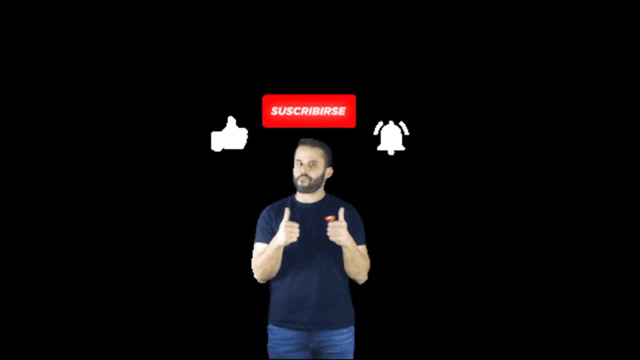 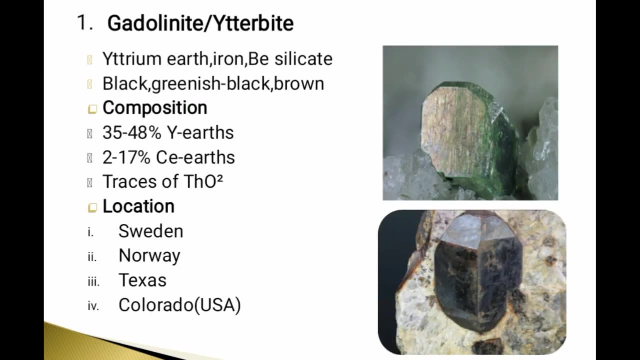 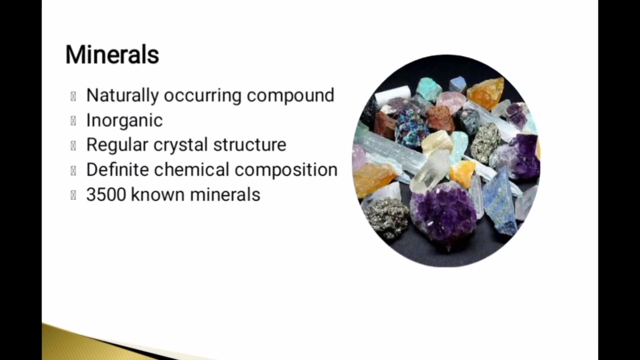 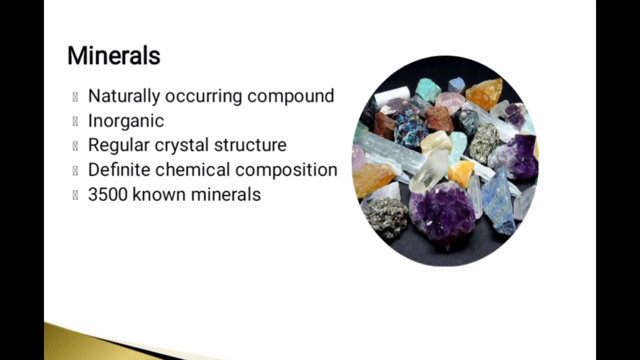 Hey, hello and assalamu alaikum. today in this video, we will discuss real earth minerals and its classification. so let's start. minerals are naturally occurring compounds which are in organic nature and they have regular crystal structure and definite chemical composition. and we also know there are literally thousands of different groups. 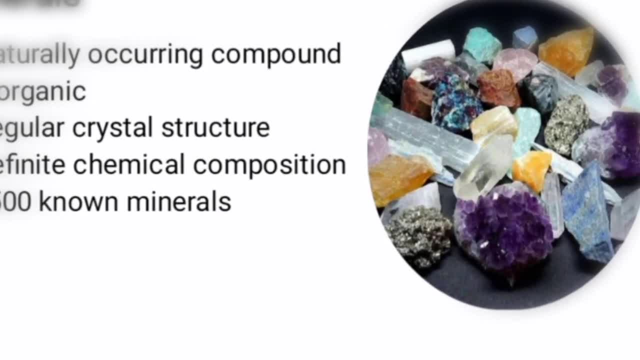 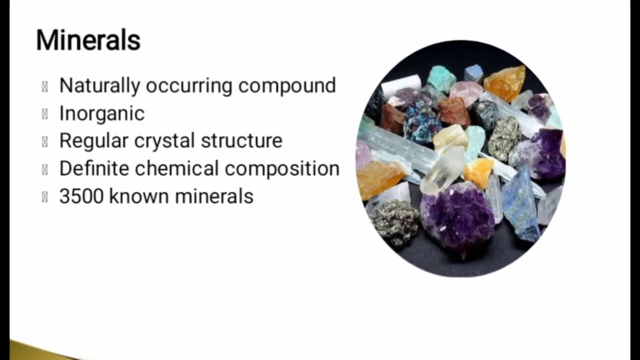 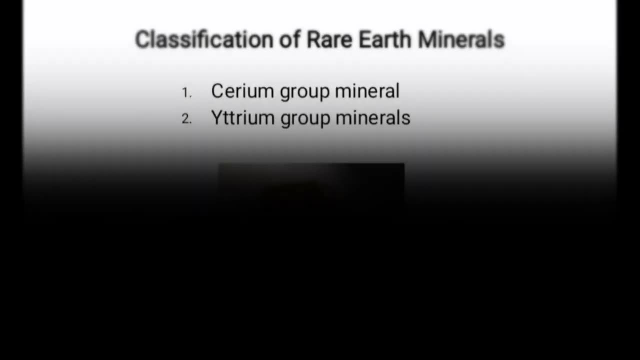 our types of minerals are present on the surface of earth, and all of these minerals have unique and interesting characteristics like color, crystal structure, even taste and smell. if we talk about the real earths, then this refers to 17 minerals which have unique and interesting magnetic and 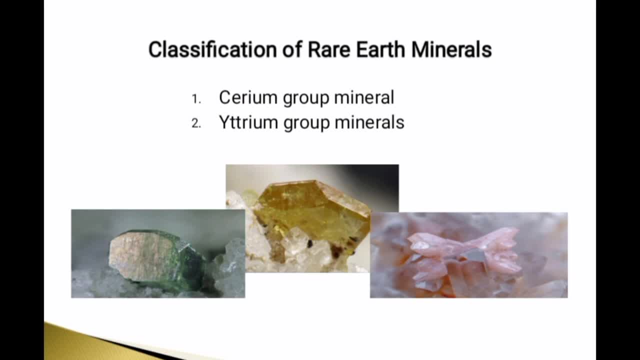 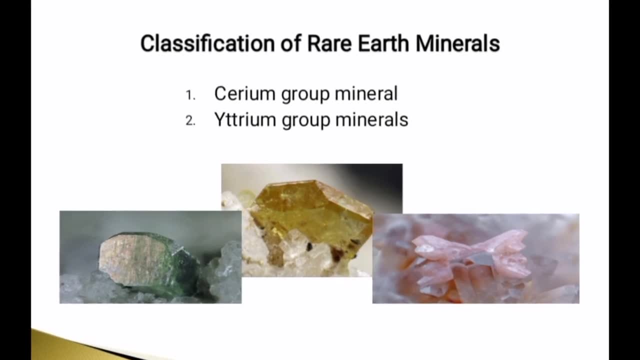 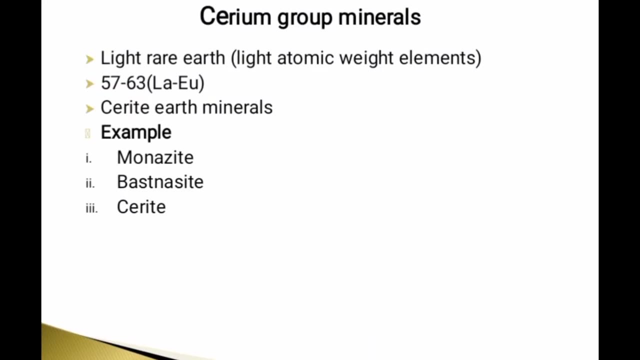 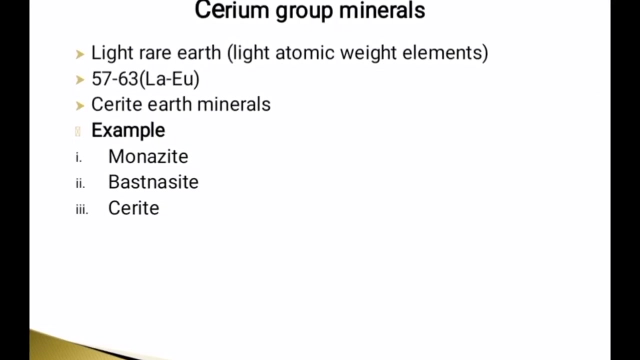 conductive properties. so if we talk about its classification, then rare earth minerals are groups. first one is serum group minerals and second is yttrium group minerals. so the first one is serum group minerals. it is also called light jurors because in it light weighted atomic elements are present, from atomic number 57 to 63 means from lanthanum to european. 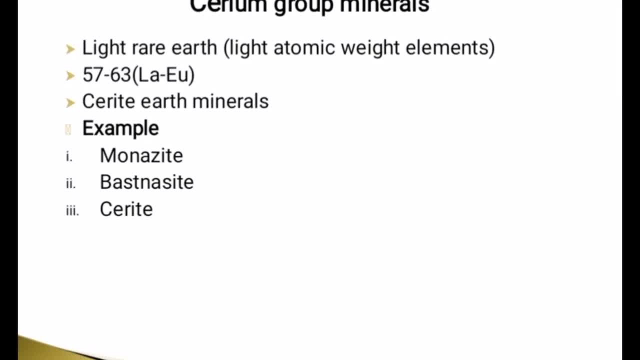 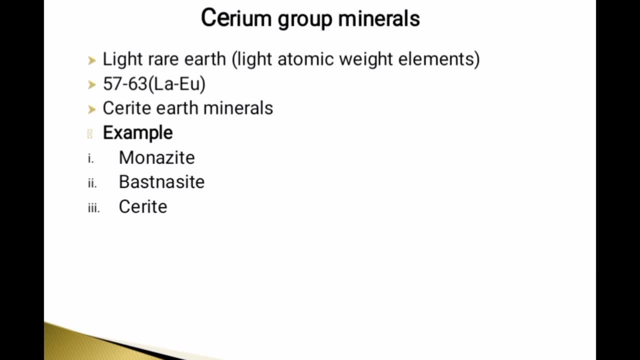 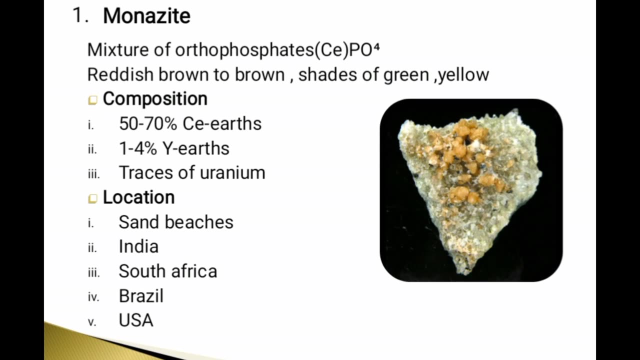 and it is also called the right rear arts or syrite earth minerals. common examples are monazite, basmosite and syrite. so the first one is monazite. it is the mixture of all the phosphates, and its color is reddish, brown to brown. 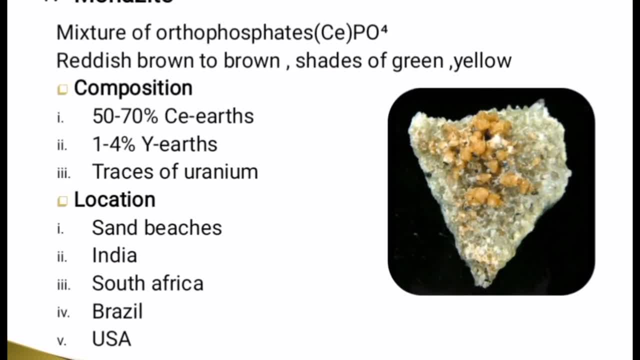 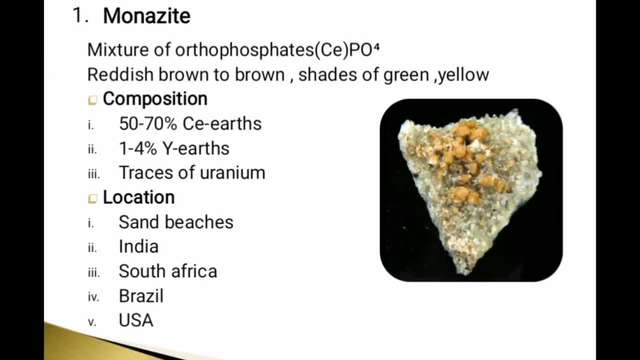 shades of green are yellow are also present. you can see here the very pretty yellowish color. if we talk about its composition, then it is made up of 50 to 70 percent ceramics. 1 to 4 pieces of uranium are also present. due to this, it is slightly radioactive, if you talk about its. 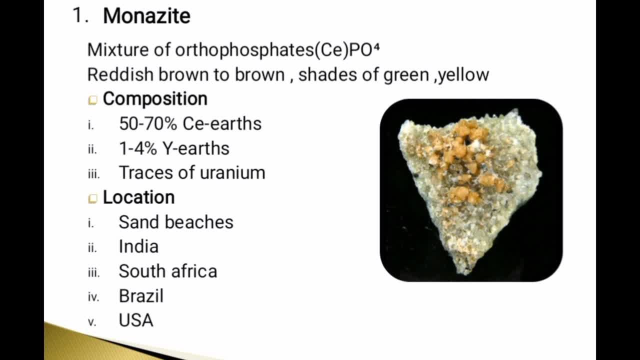 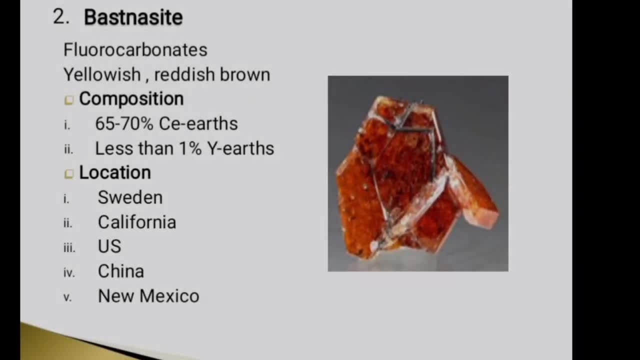 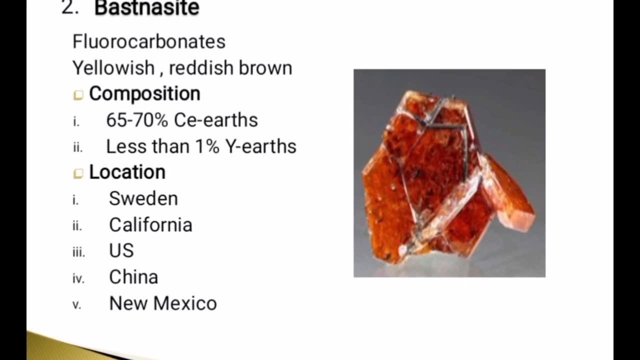 location, then it is present in sand beaches: india, south africa, brazil and usc. the next example is basman side. basically it is fluorocarbonates. it is yellowish or reddish brown in color. you can see here the very pretty reddish brown color. if you talk about its composition, then it is made. 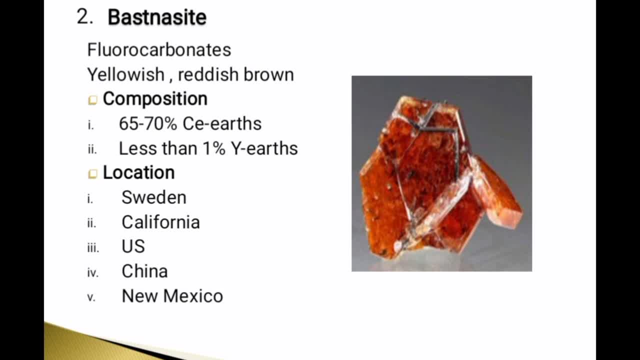 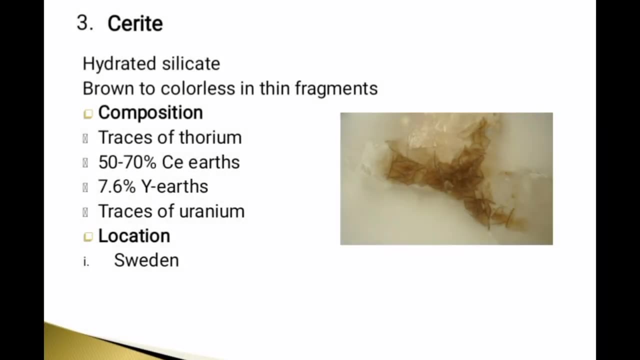 up of 65 to 70 percent cereals and less than one person get humus, and it is present in sweden, california, us, china and new mexico. next is syrite. these are hydrate silicates and its color is brown to colorless in thin fragments. if you talk about its composition, then it is made up of 50 to 70. 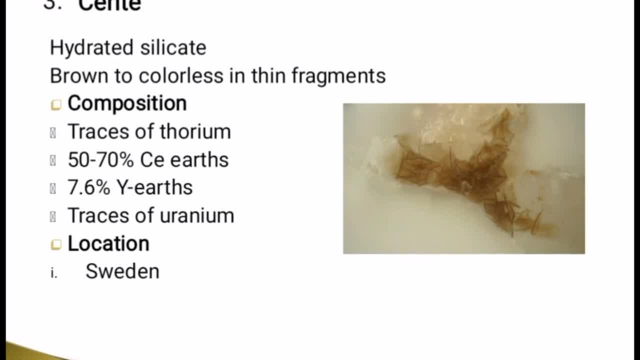 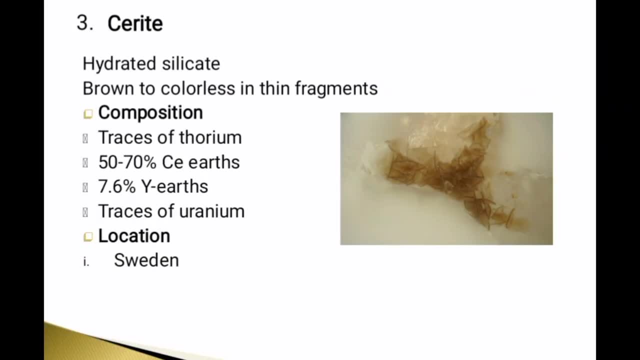 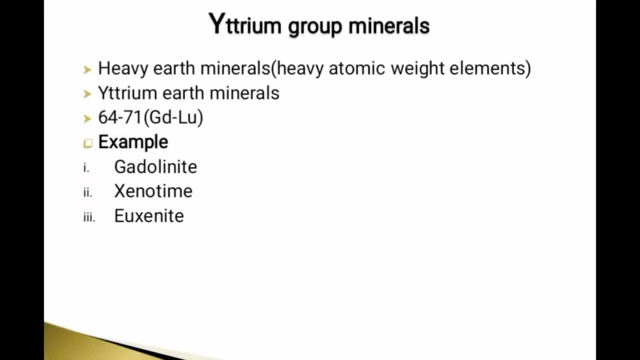 percent, cereals like monazite, seven point six percent. yet humus tracers are also present. due to this it is also slightly radioactive and it is present in sweden. the next group is yetum group. minerals basically is symbol, is capital y and its atomic number is 39 and it is also called heavy. 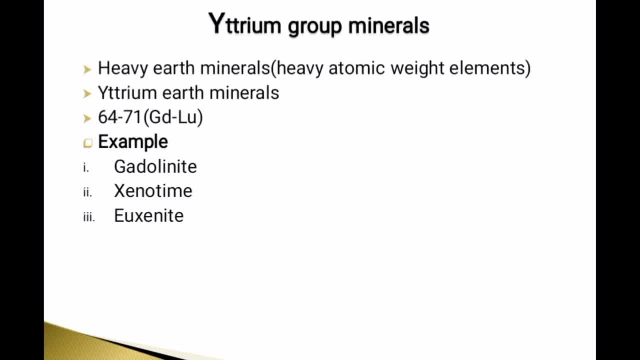 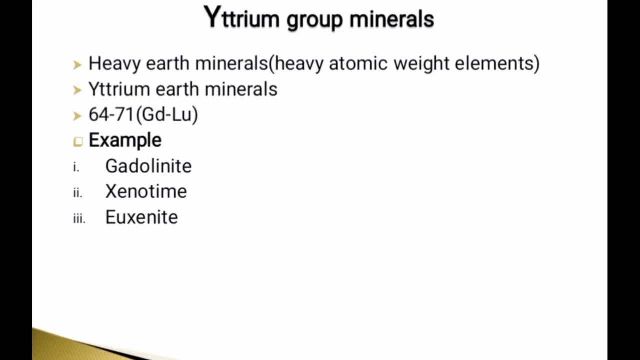 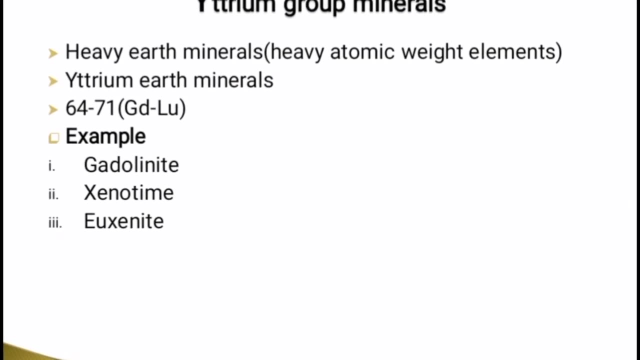 rear earths are heavy earth minerals because in it heavy atomic weight elements are present from atomic number 64 to 71, and it is also called heavy rear earths or heavy earth minerals means from gadolinium to eutresium. the most common examples are gadolinite, xenotime and. 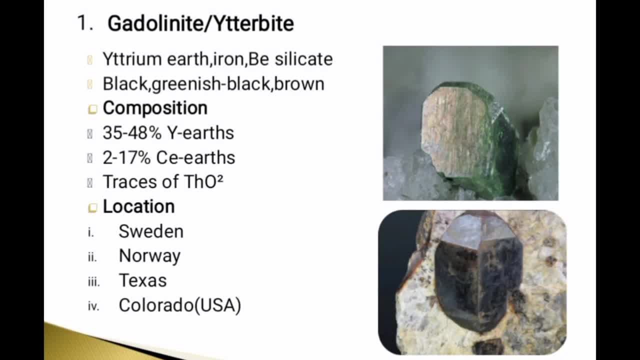 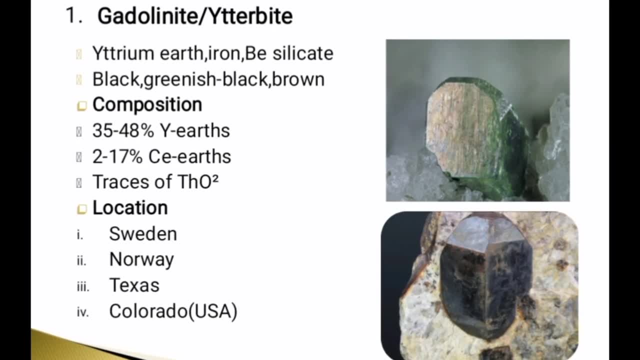 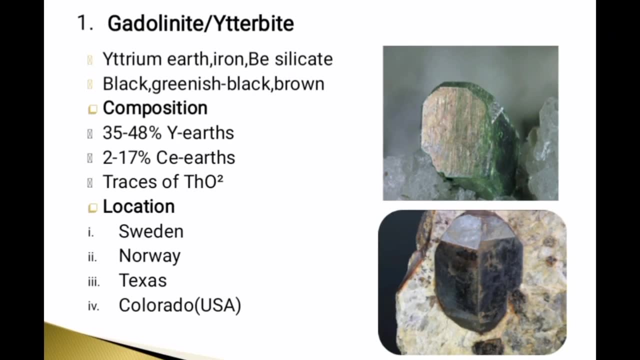 hyoxenite. so first one is gadolinite aryterbite. it is black or greenish, black or brown in color. you can see here in this picture. if we talk about its composition, then it is made up of 35 to 48 percent yet tumors, two to seventeen percent cereals and traces of thorium dioxide. 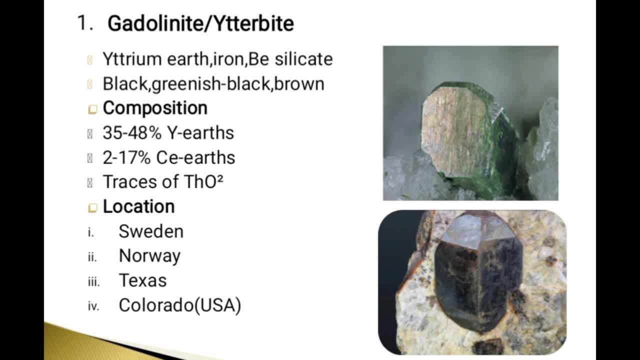 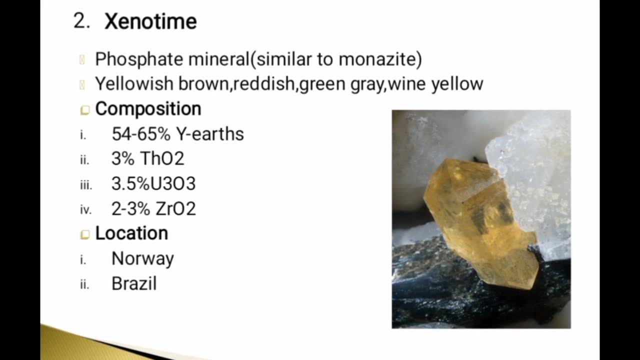 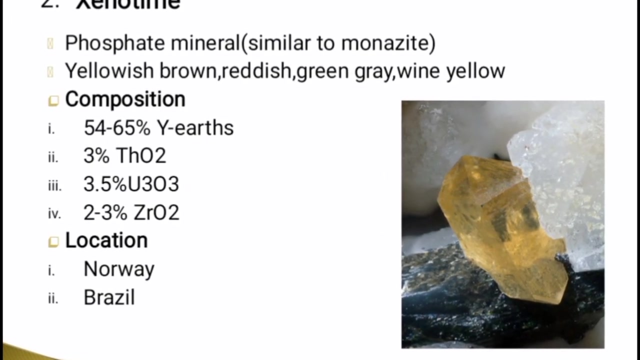 is also present. due to this, it is slightly very active and it is present in sweden, norway, texas and colorado and usc. the next example is xenotime. it is phosphate mineral like monazite. its color is for yellowish, brown, reddish, green, gray or wine yellow. it is made up of 54 to 65 percent, yet humus. that is a common disease and resp minority especially. they are useful indeed as well as to fade soil of their brethren. that is the cause of some rare leaf with arribish corona, or canadian boric inverse of varicose Benson, maybe another small species. so boric boric in Лелес, active. most are. there, foxweedo plhing东ки, is known as Conting 아마 hee them en�� inуйте, and AXs and aphrodisiac from the tof parabola, the most common is dactylje, between, and then ba na anix, slime, bridASs and and the second tri 라는. of the